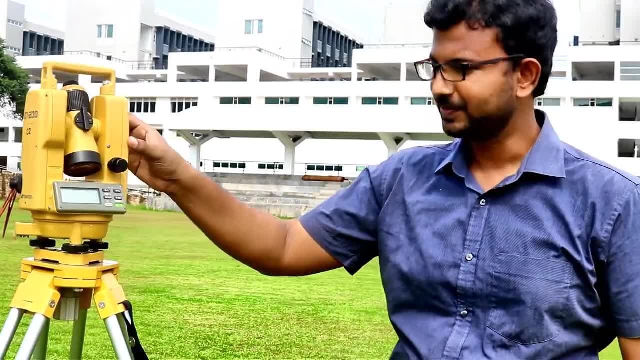 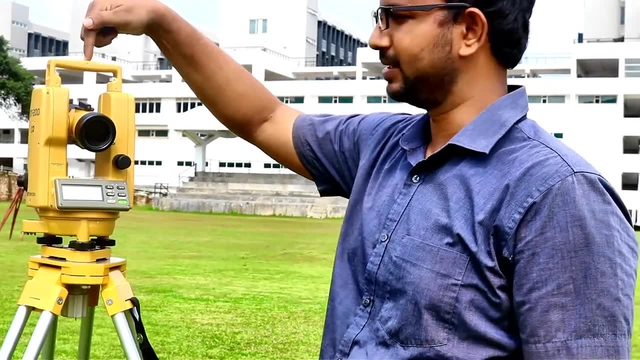 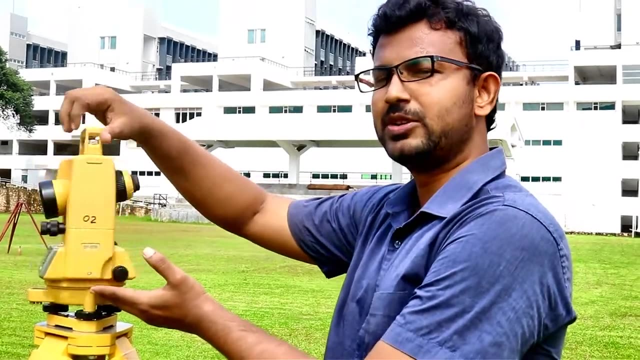 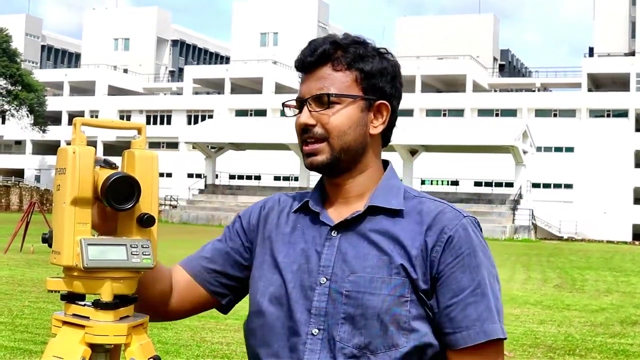 number is DT200.. The imaginary axis passing through the center of the theodolite is called the instrument axis, So the upper part of the theodolite can freely rotate about the instrument axis. It enables us to measure horizontal angles, and this telescope is pivoted above the trunnion. 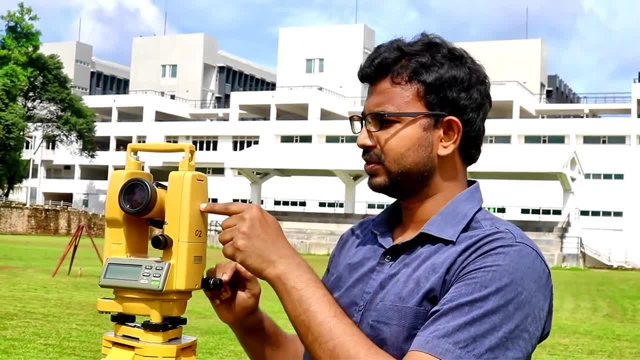 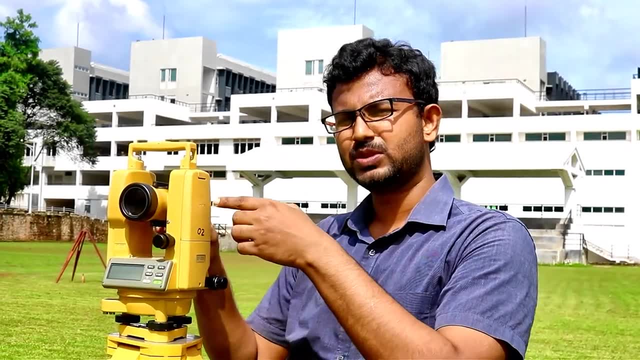 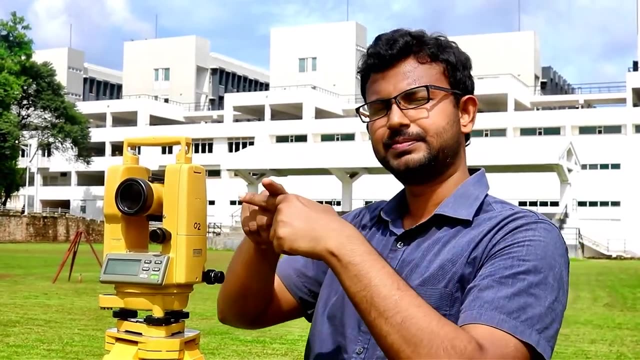 axis. The trunnion axis is the axis which passes through the center of the telescope in the direction perpendicular to the line of sight of the telescope. So the telescope is pivoted above the trunnion axis, So it enables us to measure vertical angles. 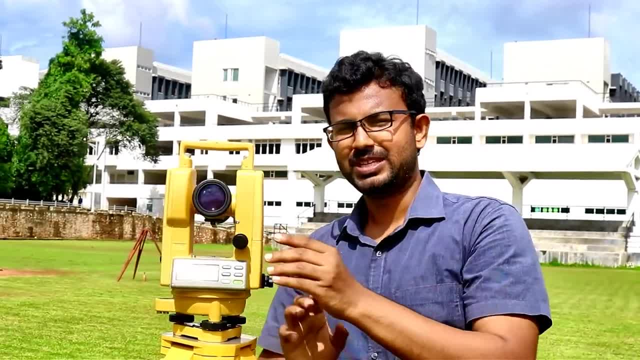 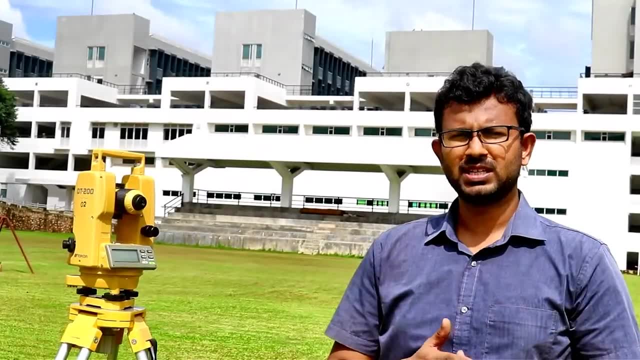 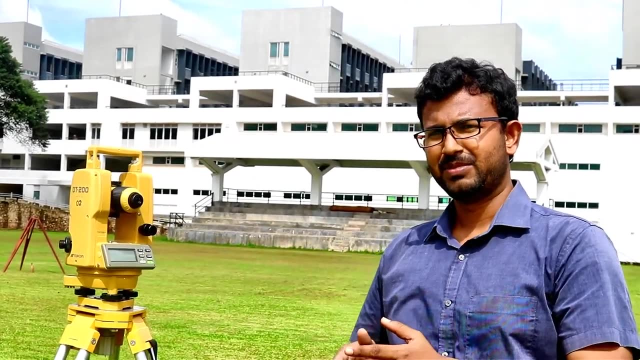 So these are the two main basic functions of the theodolite: Measuring horizontal angles and measuring vertical angles. All the other functions, just like extending a survey line, setting out 90 degrees, setting out a curve and measure a height difference, setting out. 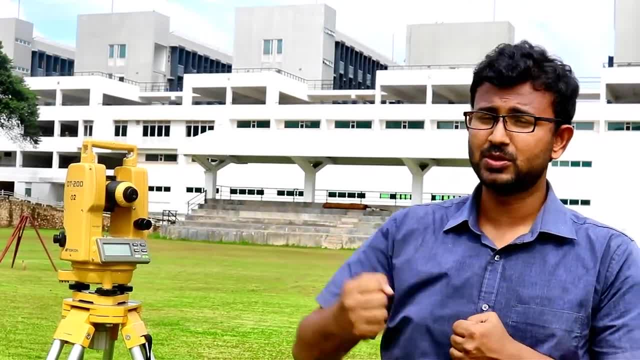 building edges, setting out the distance between two points, which is known as the tachymetric survey. I will explain in the future lessons. Right, All these are the two main basic functions of the theodolite Measuring horizontal angles. 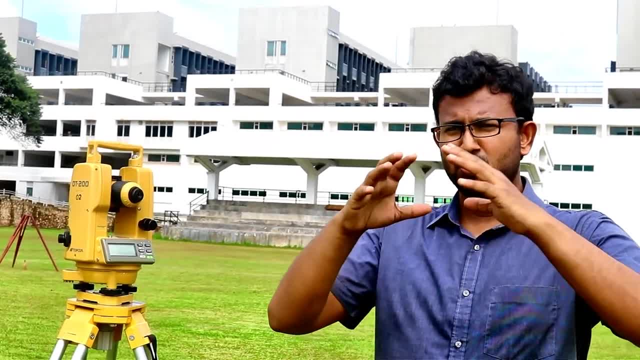 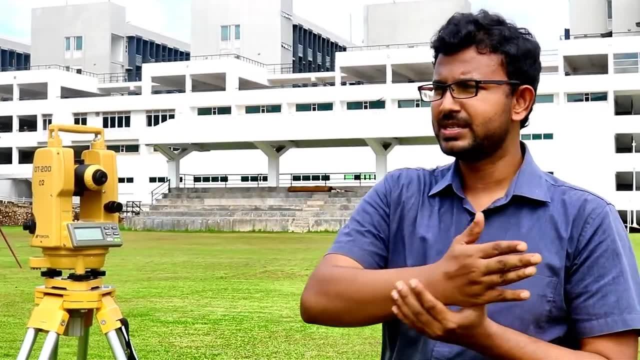 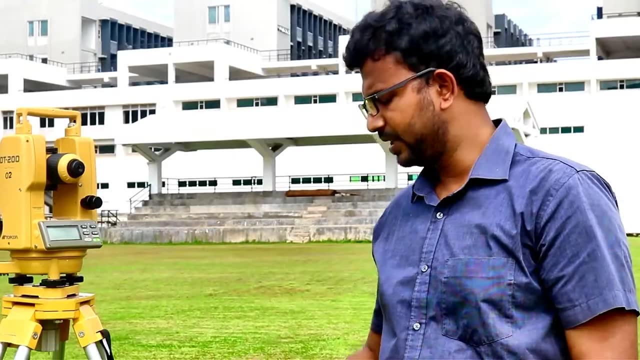 and measuring vertical angles. All are based on these two basic functions of measuring horizontal angles and measuring vertical angles. Now we will see how to perform one of the basic functions of the theodolite, that is, measuring horizontal angles. As you see, this theodolite has been fixed over this ground point. Let's take it as point. 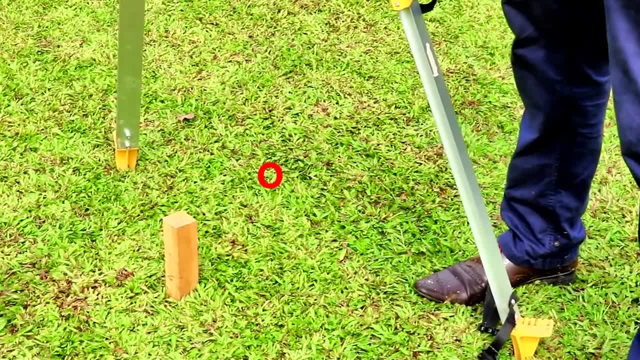 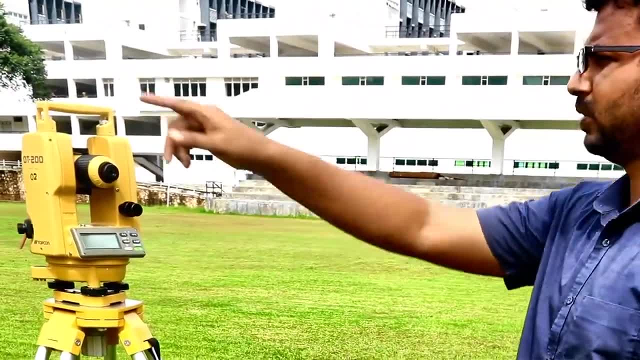 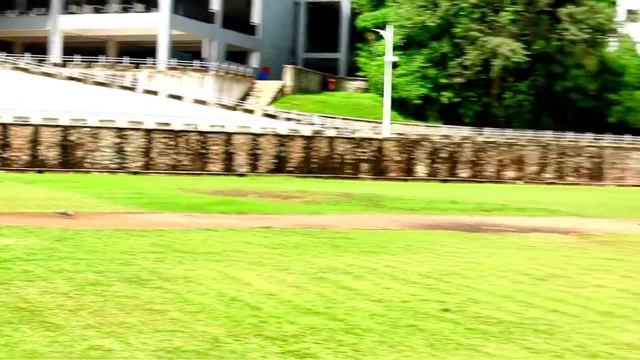 O Right, Further, I have one more thing to tell you about the theodolite Further. I have fixed one point over there. It is called point A And I have fixed a dummy there with the help of plumb box. So if you want to target to point A, what? 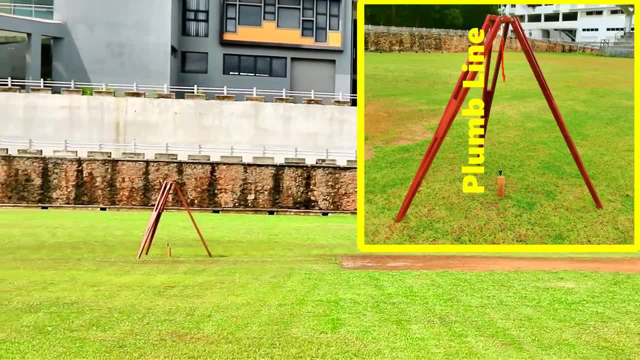 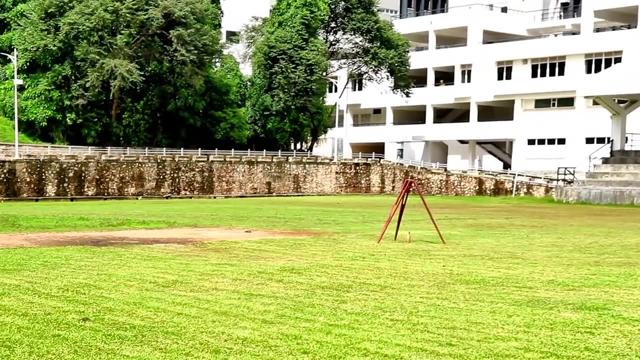 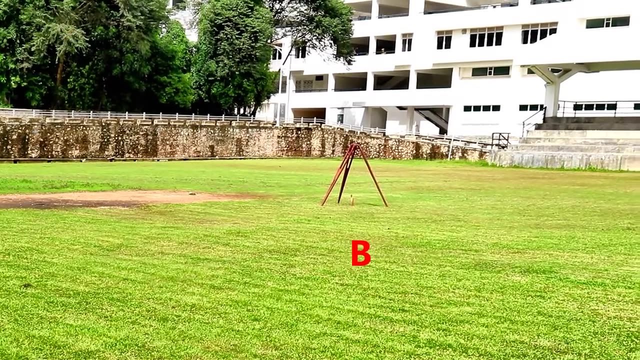 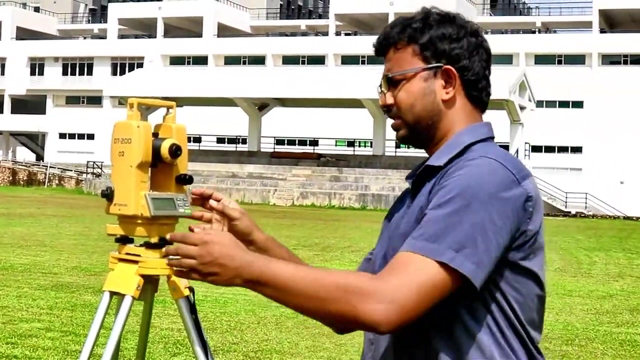 you need to do is you need to target to the plumb line, And I have fixed point B over there. Similarly, I have fixed a dummy over there And, with the help of plumb line, we can target to the point B Right Now. we'll see how to. 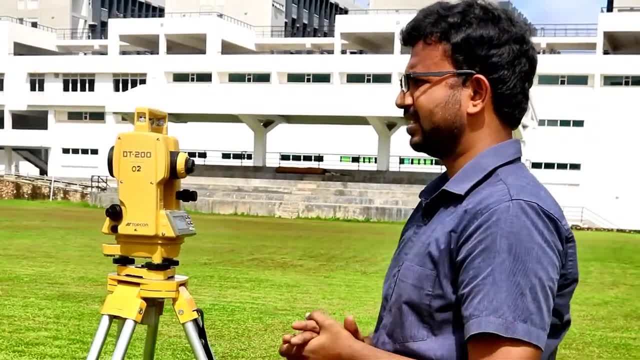 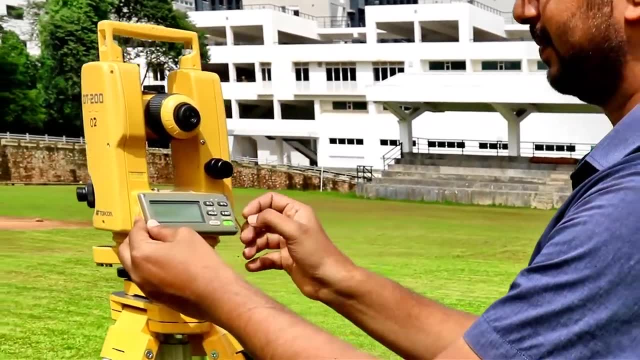 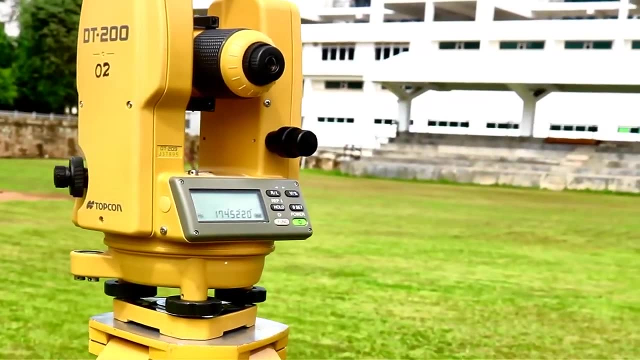 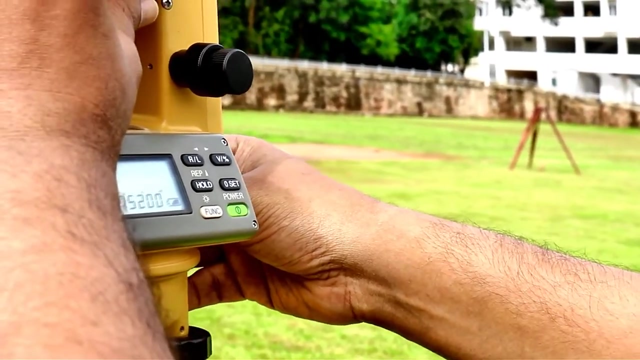 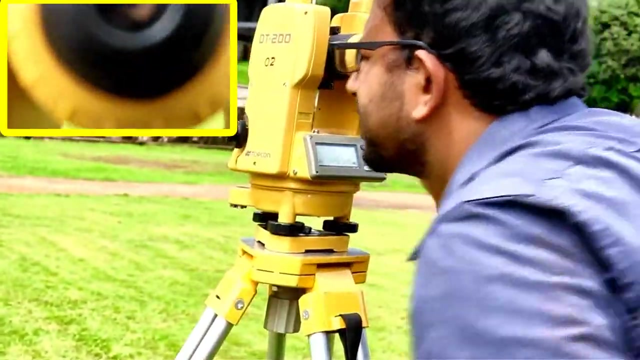 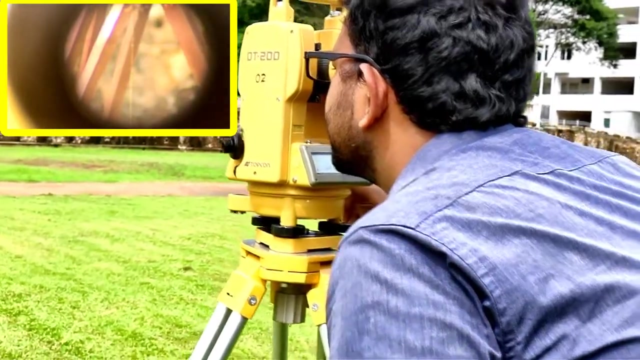 operate this instrument in such a way that we can measure horizontal length Right. Right Now. I have switched on the instrument. Now what I'm going to do is I'm going to target, to point A Right When you are targeting Right. 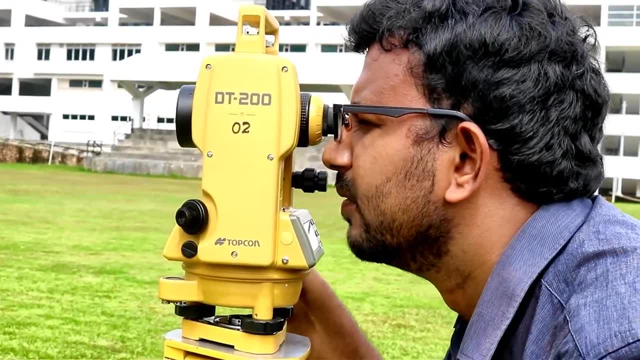 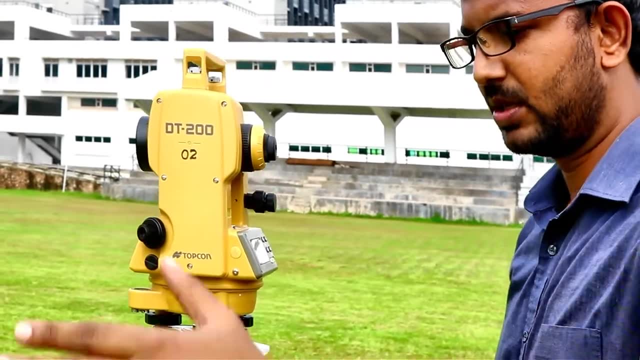 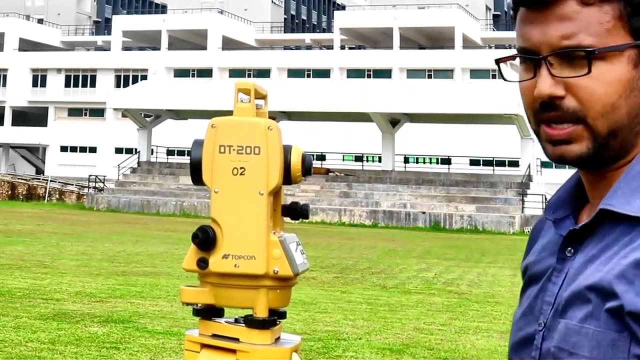 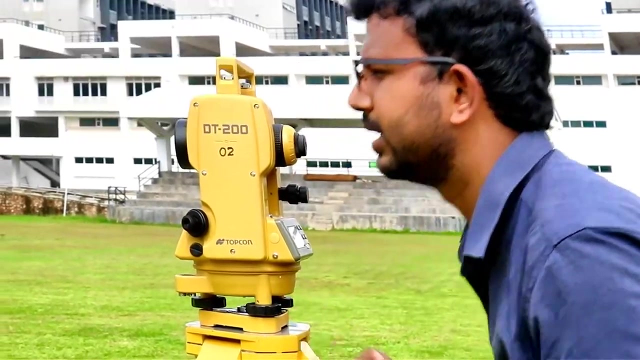 Right, Right, Right, Right. to point a, it's better to target to the top of the plumb line because the bottom part swing here and there due to the wind right, so moments are less in the top part of the plumb line. so now i have already targeted to point a. 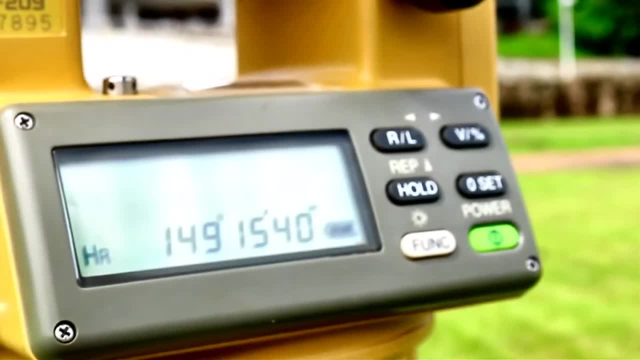 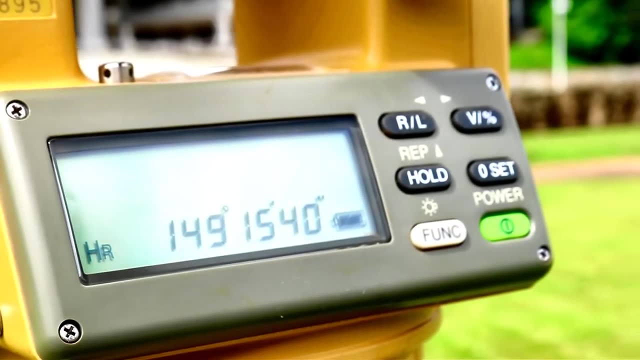 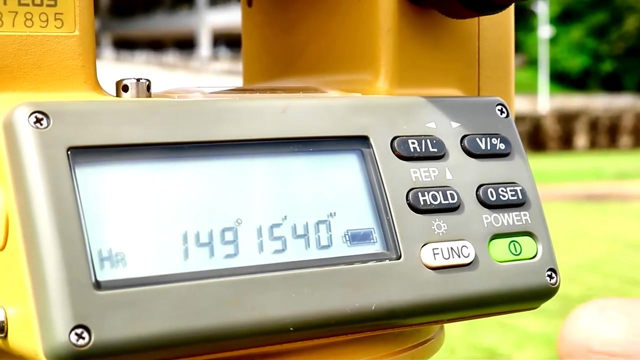 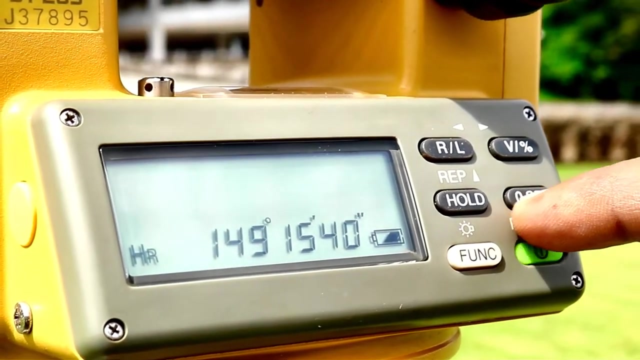 the shown angle is 149 degrees, 15 minutes and 40 seconds. so here it shows the horizontal angle of point a, right. so what we need to do is we need to set the zero to the point a. for that we can use this offset offset button. once you press it twice. 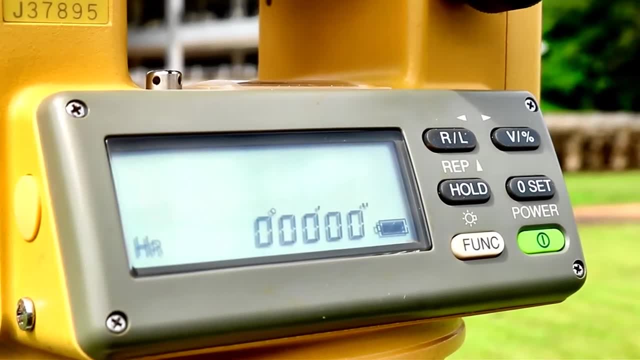 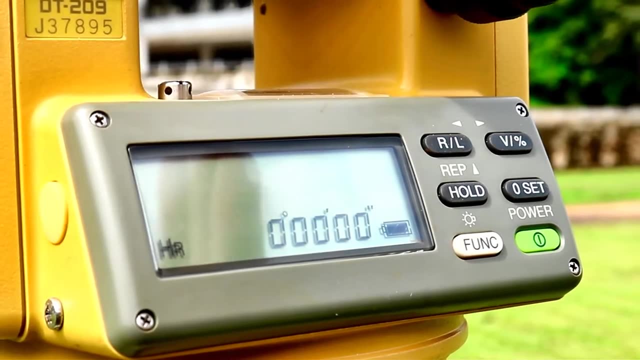 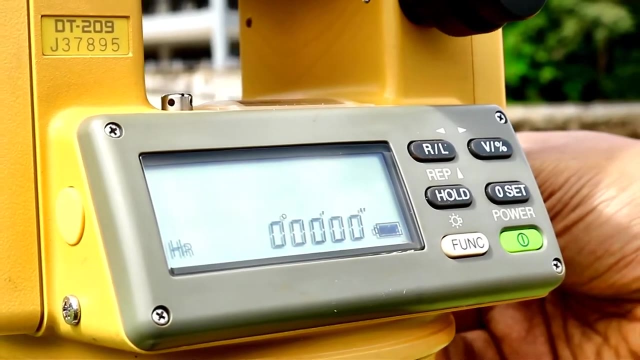 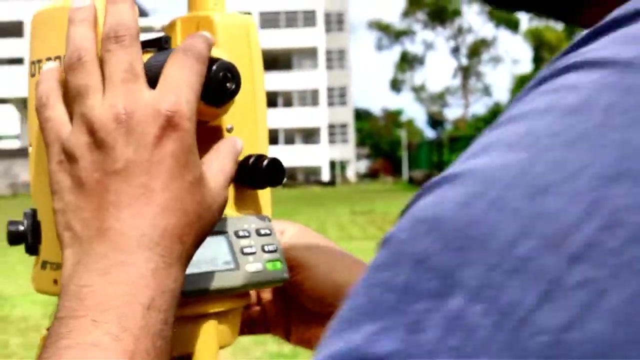 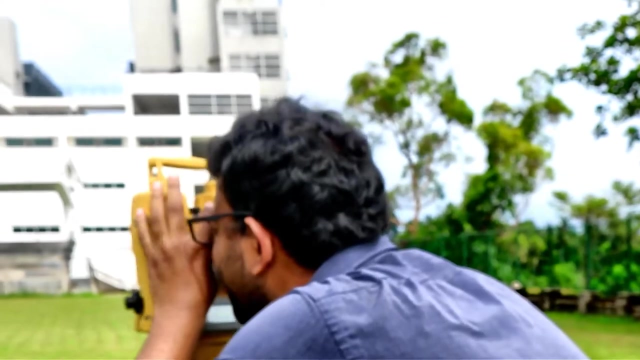 the angle is set to point a and the angle becomes zero to point a. then it helps us to get the direct bearing to point b from point o, where the instrument is right. so now i'm going to turn the instrument. now you see, the angle increases. now i'm going to target to point b. 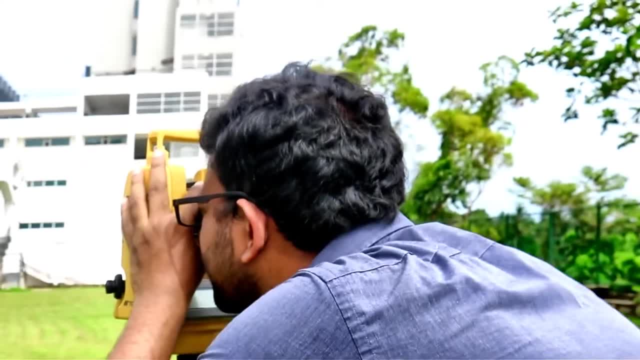 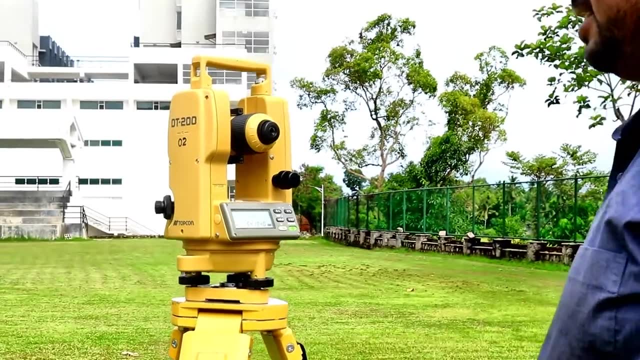 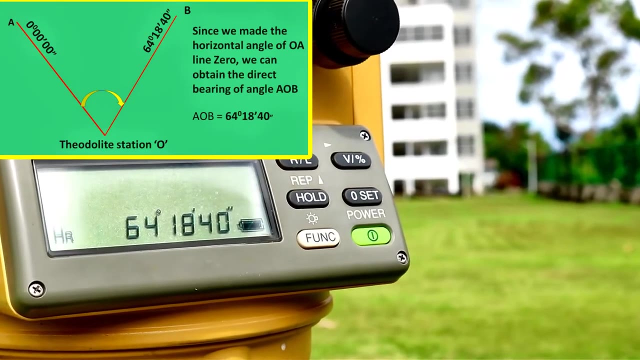 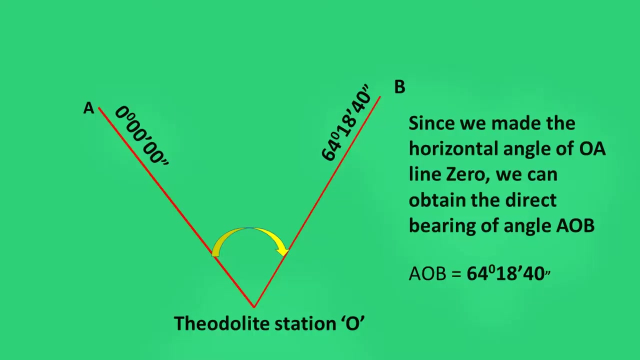 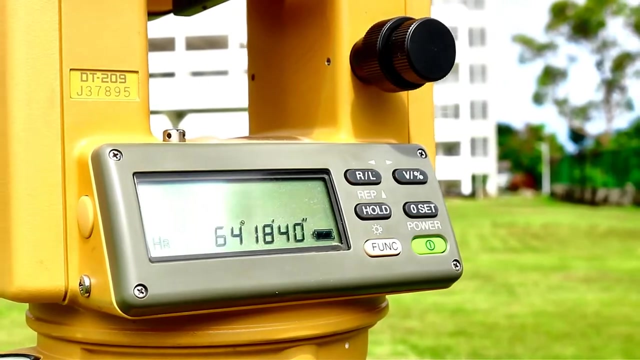 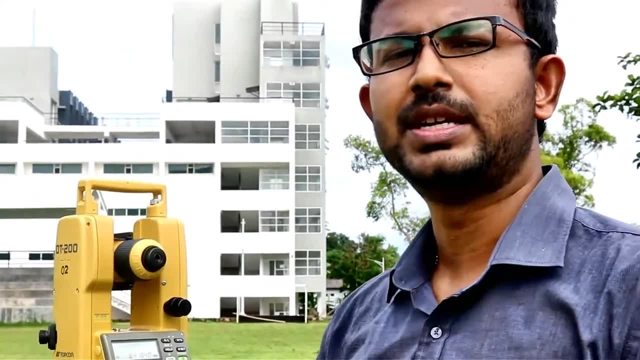 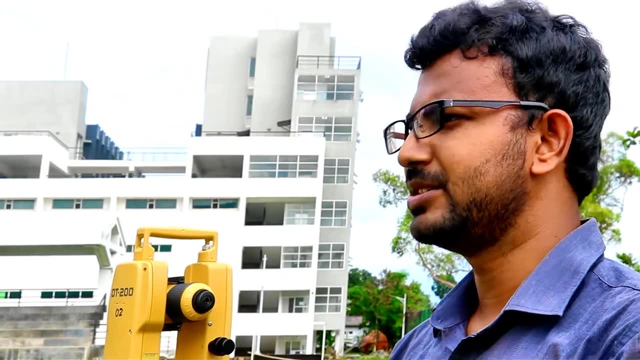 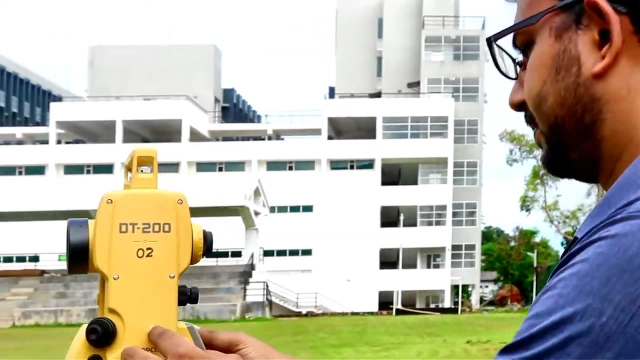 the direct bearing from point A to point B, that is, 64 degrees, 18 minutes and 40 seconds. if you don't have that option setting zero, what you can do is you can record the angle to point A. right, let's do that as well, right. 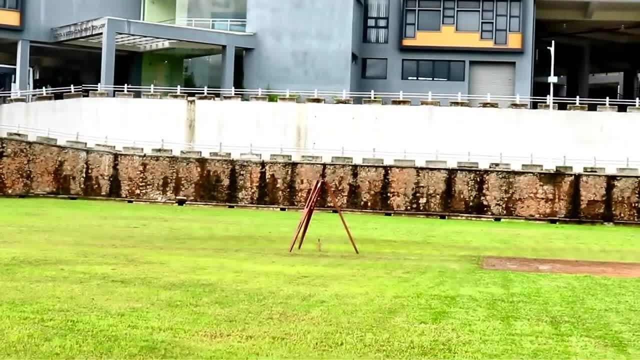 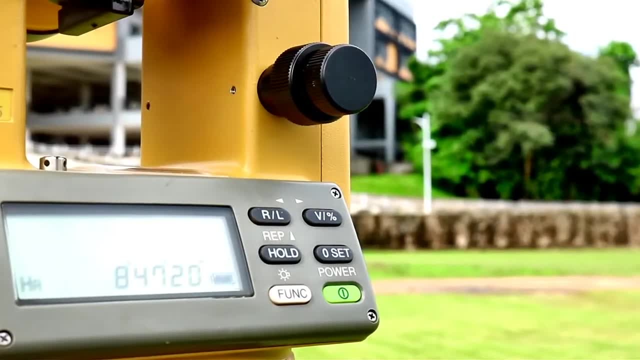 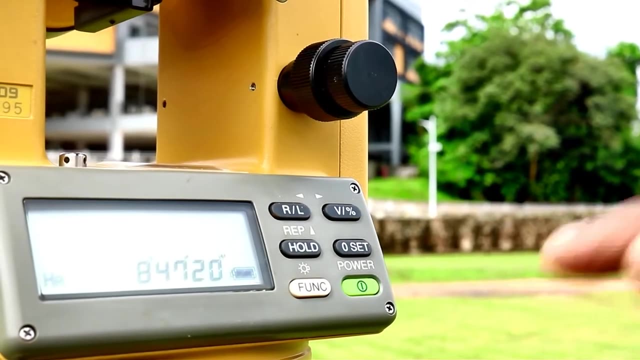 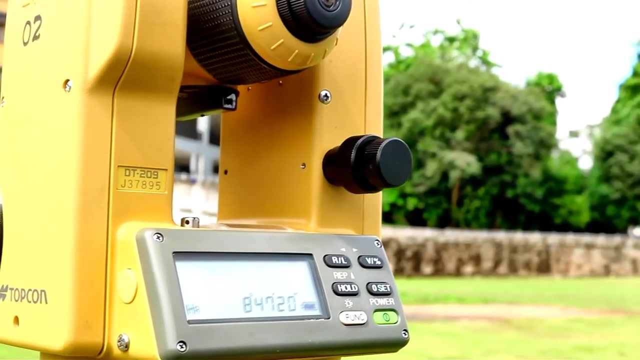 now I have already targeted to point A. the shown angle is not the zero right. it is 8 degrees, 47 minutes and 20 seconds. now you need to record or note down this angle: 8,, 47, 20. then what you have to do is you don't need to set zero right you. 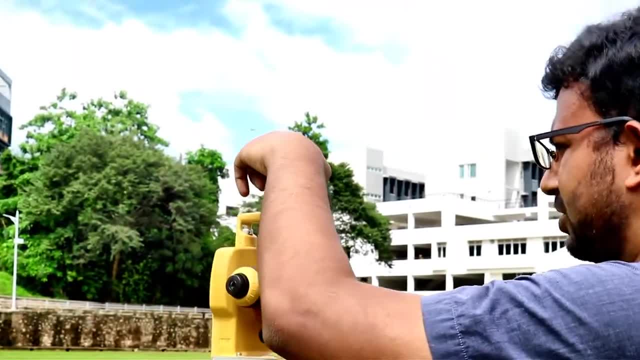 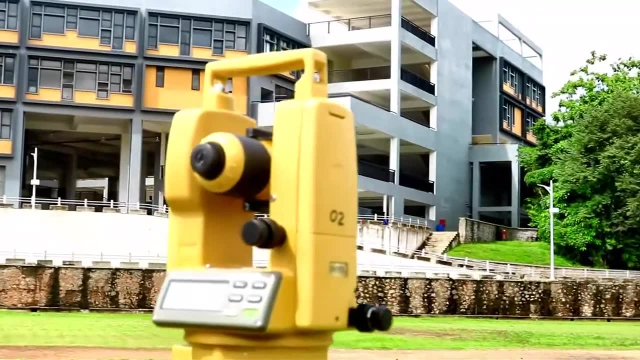 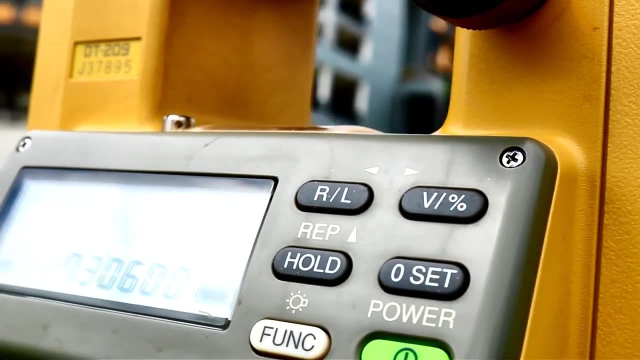 need to set 0.. to turn the telescope about the instrument axis and target back to the point B. the angle is 73 degrees 6 minutes and 0 seconds and you need to note down this angle aspect right if you deduct the previous angle from this. 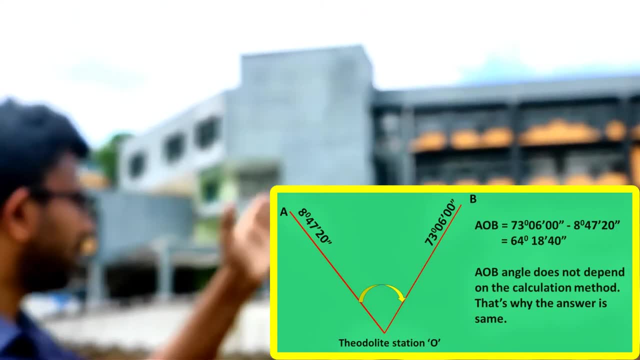 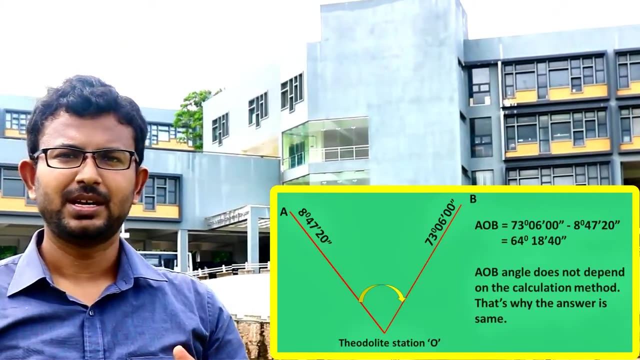 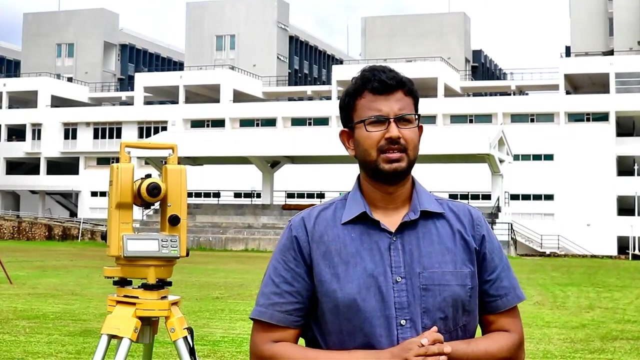 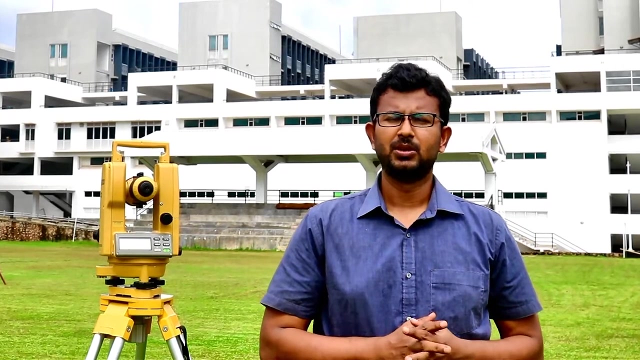 angle. you will get the angle from point A to point B measured from point O right. so that is how we can measure a horizontal angle. now I will explain the uses of measuring horizontal angles. in surveying we have to establish control points which have known coordinates. we call them northern, easting and southing coordinates. 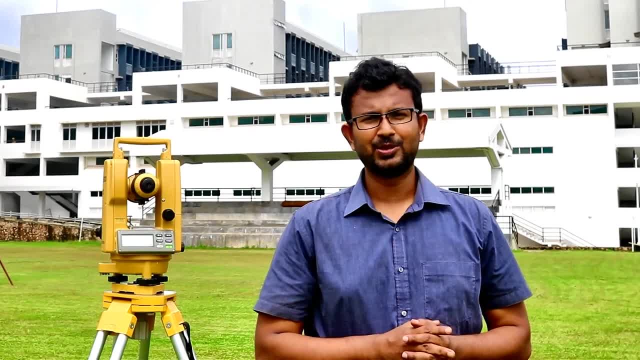 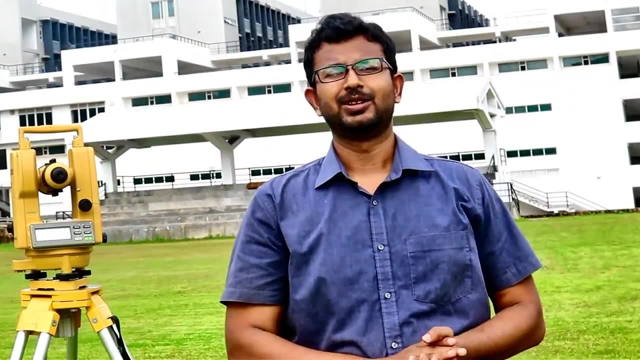 in your A Levels you know that there are three coordinates called X, Y and Z. here in surveying you have three coordinates. those are known as northern, easting and southing coordinates. The coordinates used are xyz and z. the north direction are called northing coordinates. coordinates in the east direction are called 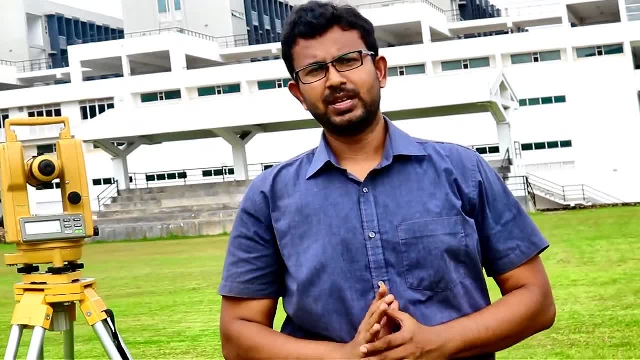 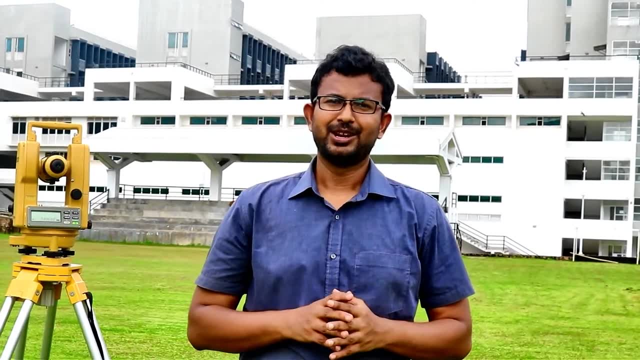 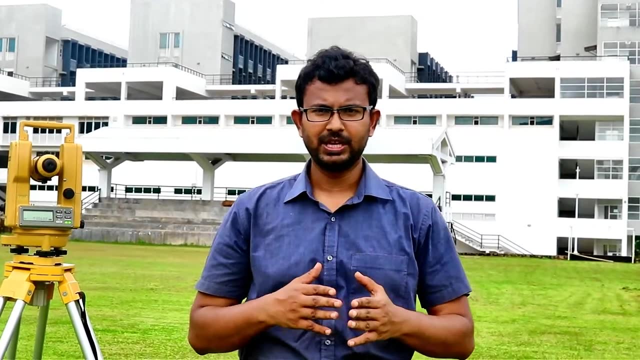 easting coordinates and z coordinates is the height. right control points are the points which are having non-northing easting and zenith coordinates. so northing and easting coordinates are calculated with the help of the length of a traverse leg and the bearing to the traverse leg. 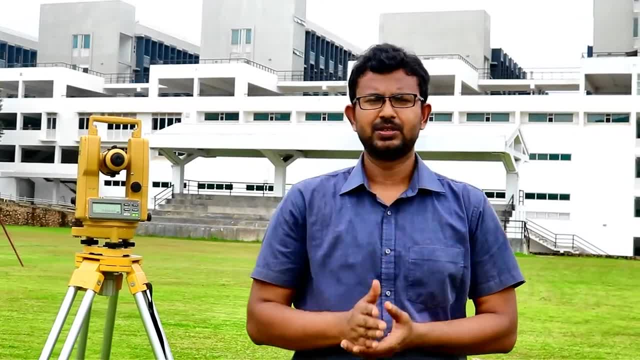 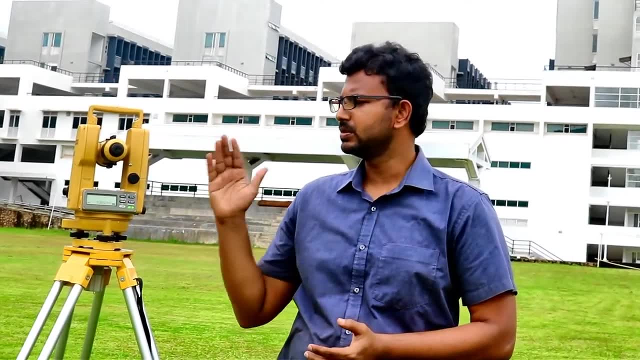 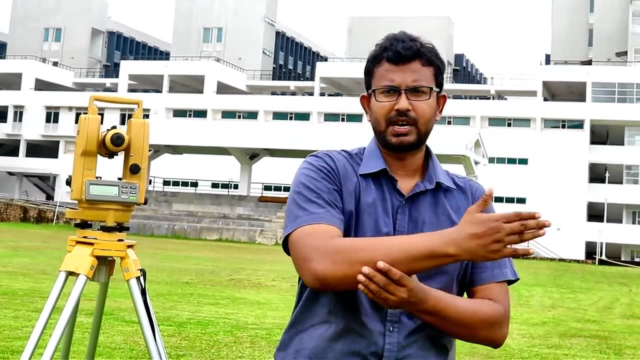 from the north. the bearing to the traverse leg should be measured from the north or should be measured from another traverse leg. so for that we have to use this teodolite right. so from the teodolite we can measure the bearing between two legs of a traverse to obtain that horizontal angle. 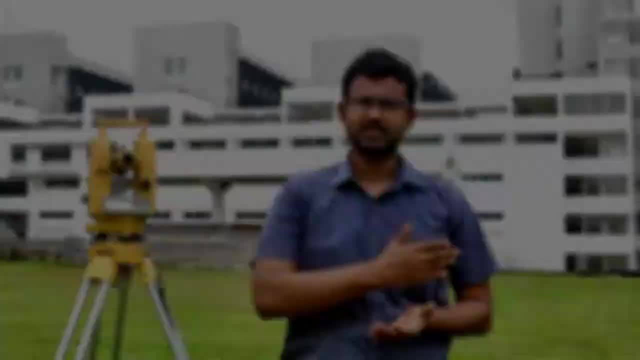 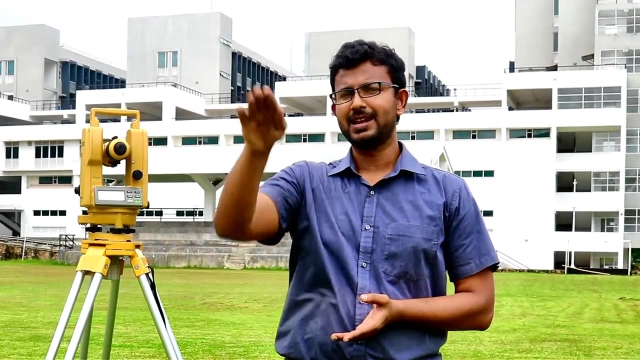 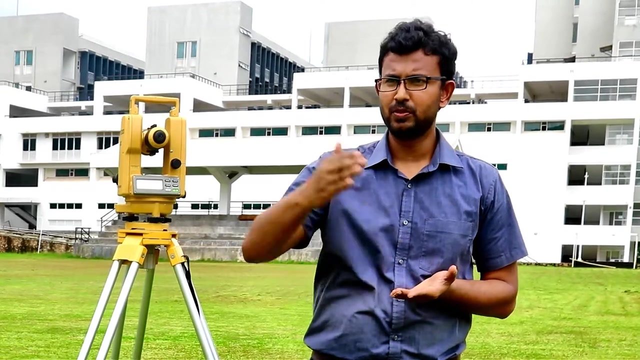 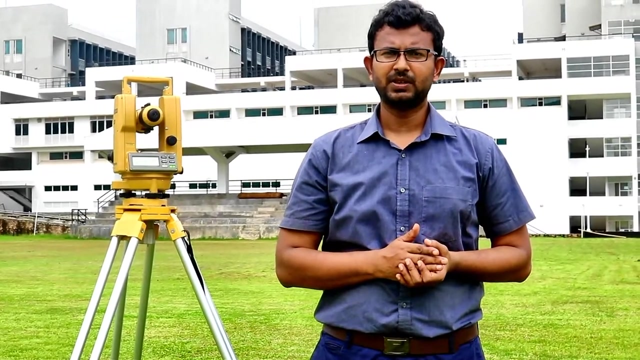 we have to use the digital or other type of teodolite. the next basic function, the measuring a vertical angle, is used to measure a slope in a land, to find out a height difference and to find out the distance between two points using the tachymetric survey and etc. now we will see how to measure a vertical 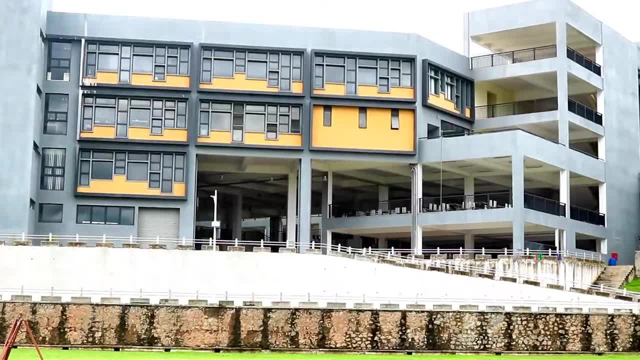 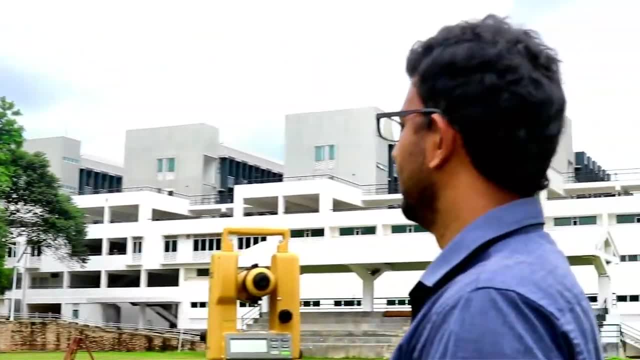 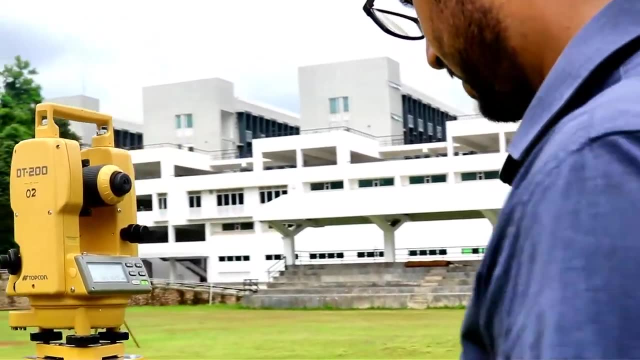 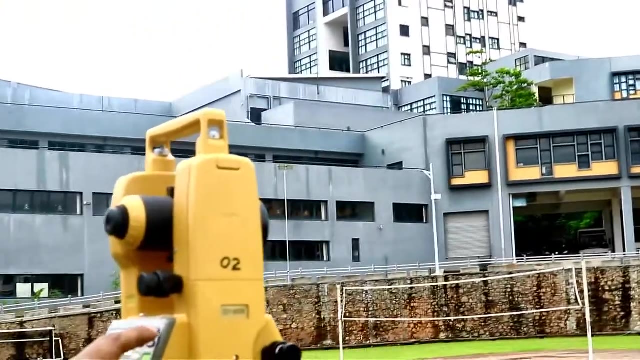 angle between two points right. so angle between the top of the building and the top of the handrail can be measured using the teodolite. this is how i am going to do that. first i switch on the teodolite, then now here it shows only the horizontal angle right. what i have to do is i have to press v. 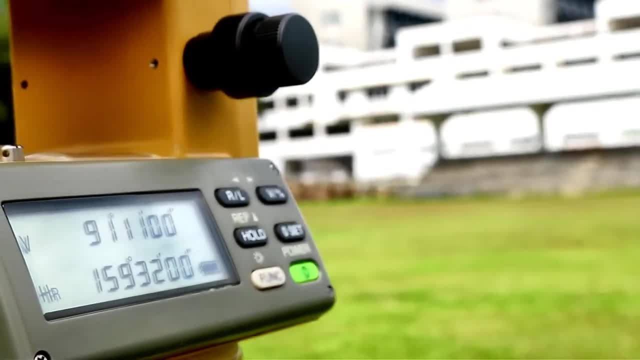 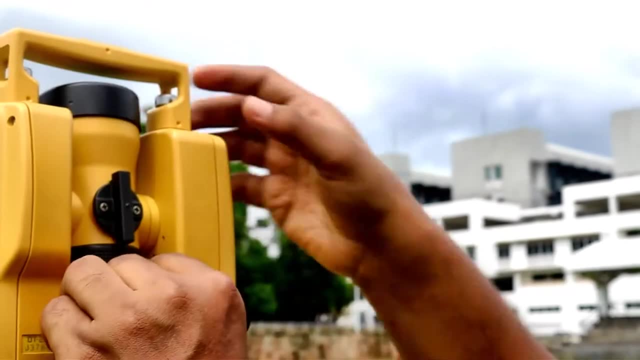 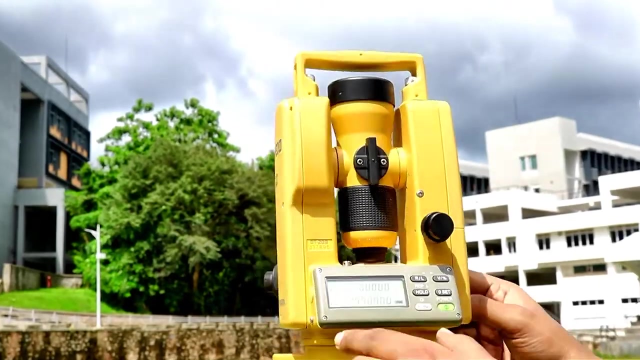 then it shows the vertical angle. now the vertical angle is 91, so vertical angles are normally measured by the vertical angle and the vertical angle is 91.. and the vertical angles are normally measured from the zenith axis. zenith axis is the instrument axis and now, you see, the vertical angle becomes zero. 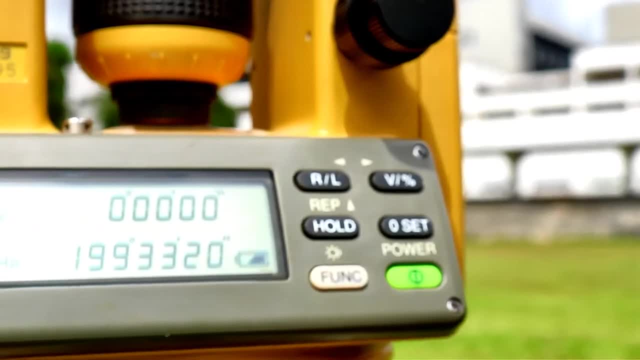 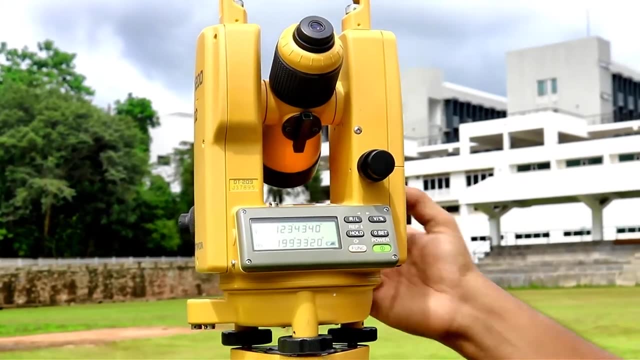 when the telescope is held upright. when i depress the telescope, angles are increasing. so now we'll target to the top of the building. we'll see the angle between the two огромード e길 garbage point and we will also measure on top of the building. 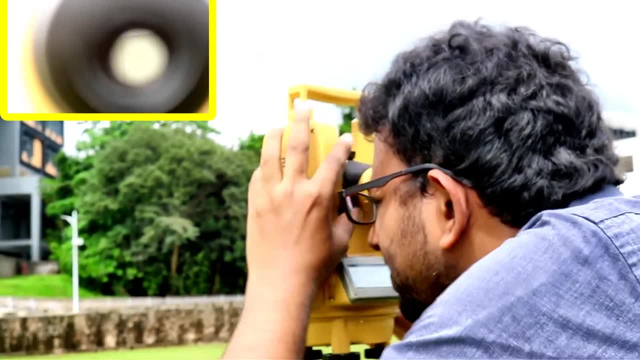 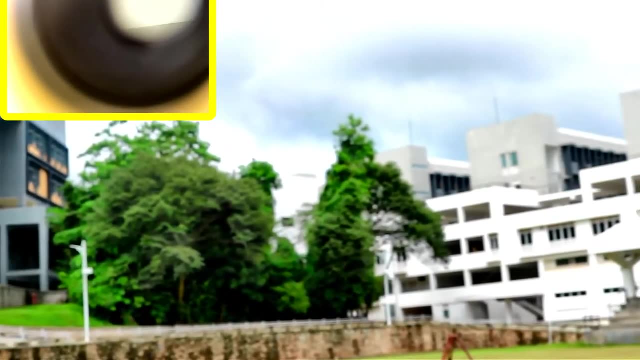 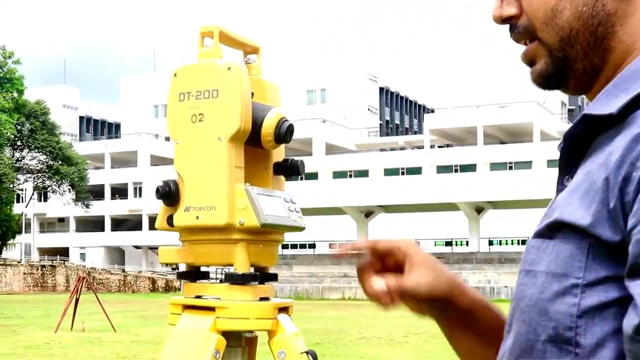 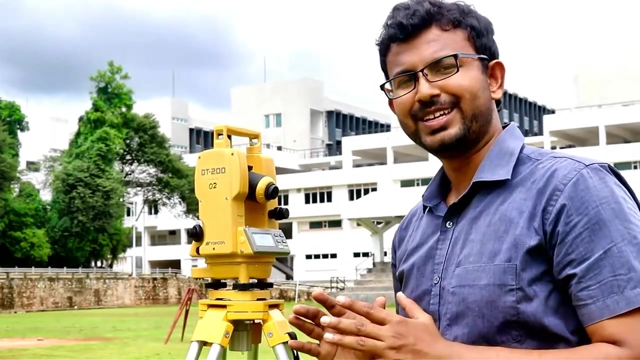 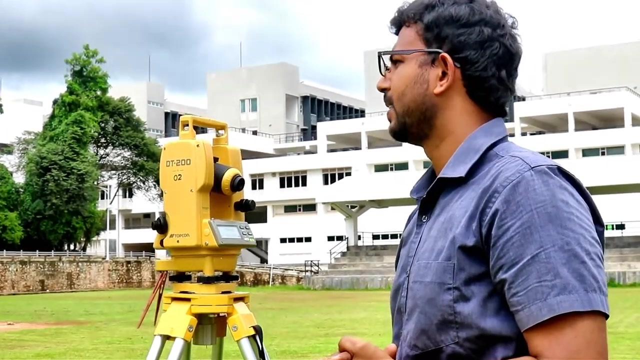 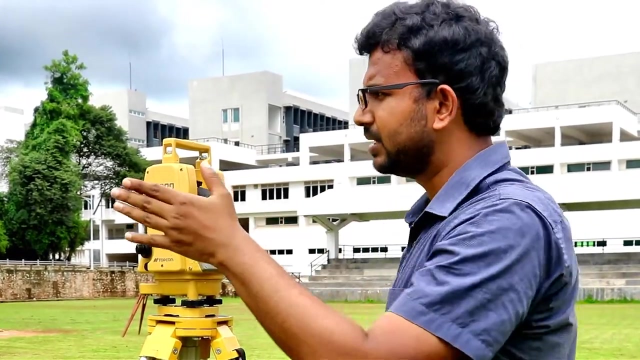 the angle from zenith to the top of the building right. the angle is 73 degrees 4 minutes and 0 seconds. that is how we can measure the vertical angle to any of objects. not only that, we can measure the vertical angle difference between two objects, as I explained before for the horizontal angle measures right. so 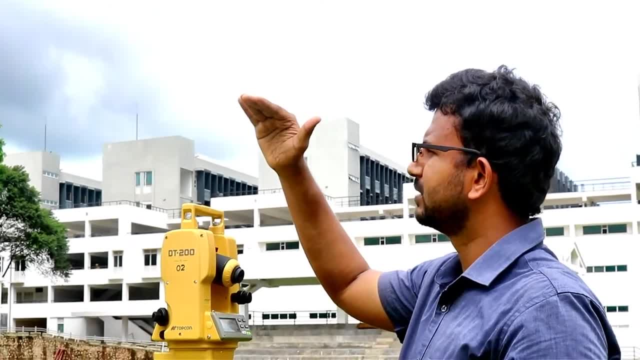 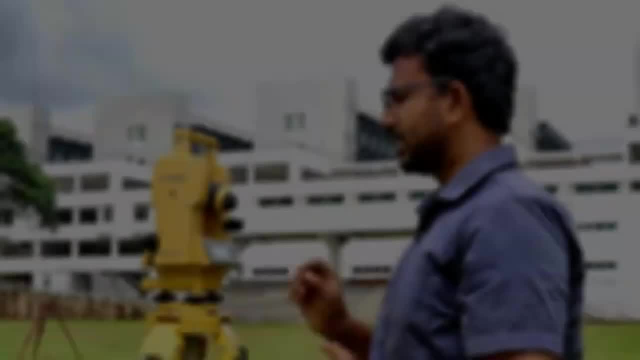 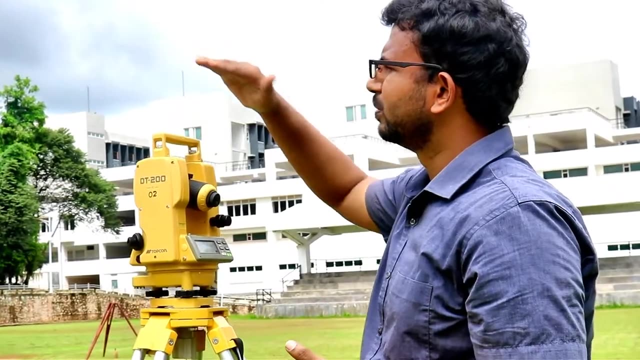 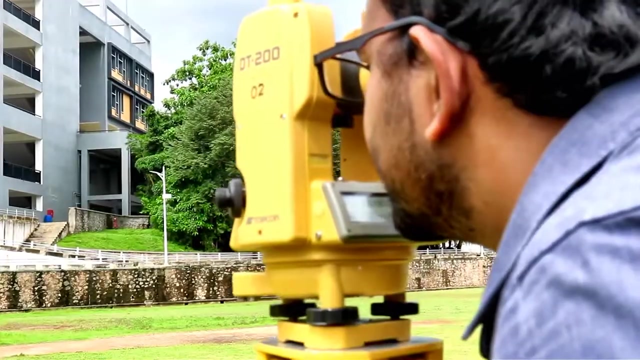 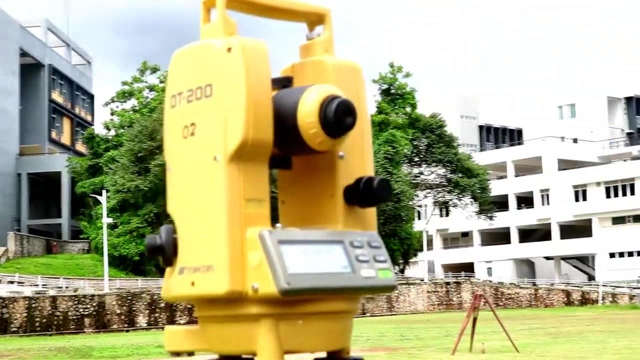 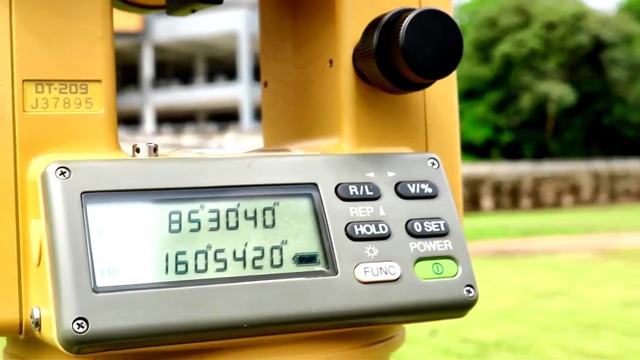 if I want, I can find the angle difference between the top of the building to the top of the right. what I have to do is I have wrote down this. I have already targeted to the top of the handrail. the vertical angle is 85 degrees, 30 minutes and 40 seconds right if you deduct the previous reading. 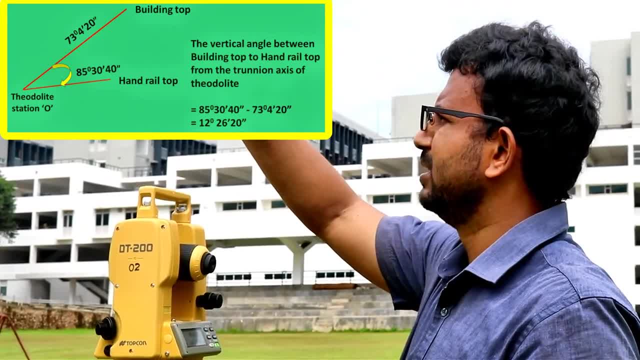 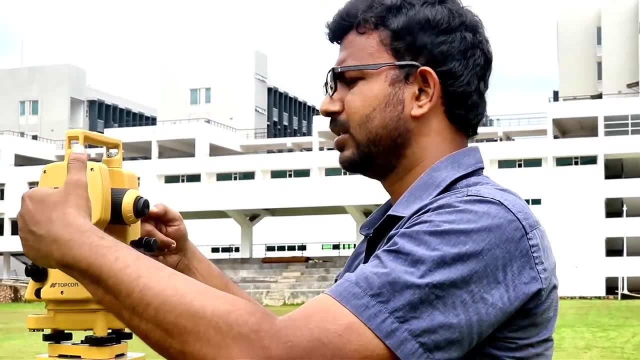 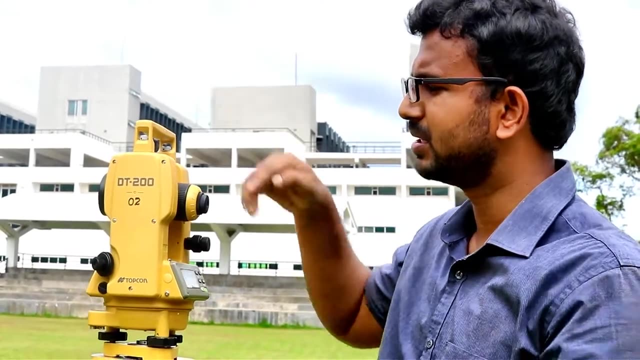 from this reading. you will get the angle between the top of the building and the top of the handrail from the trunnion axis. the telescope is pivoted about the trunnion axis. therefore, whatever the vertical angles you measure is measured, referred to the trunnion axis. so trunnion axis is the center of the angle. 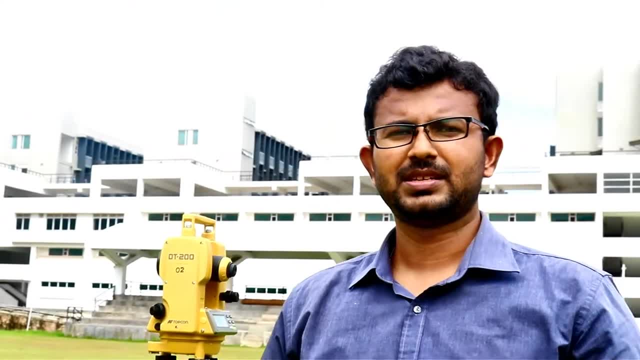 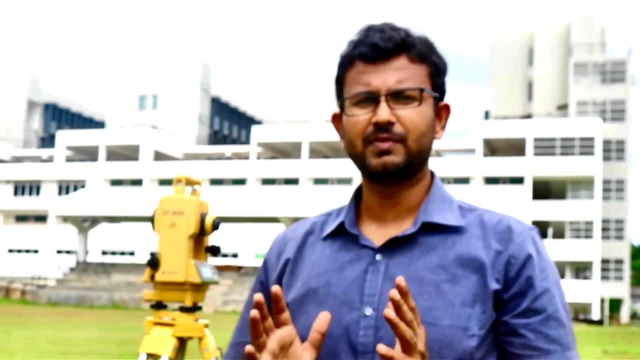 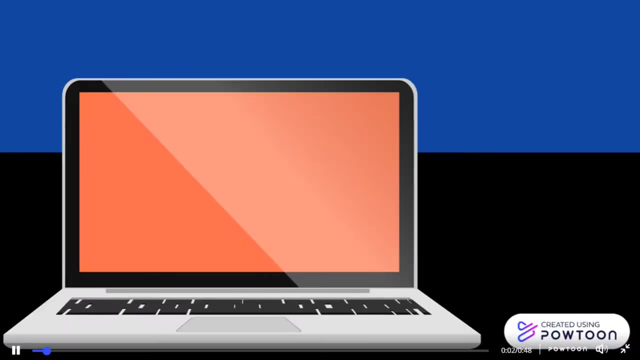 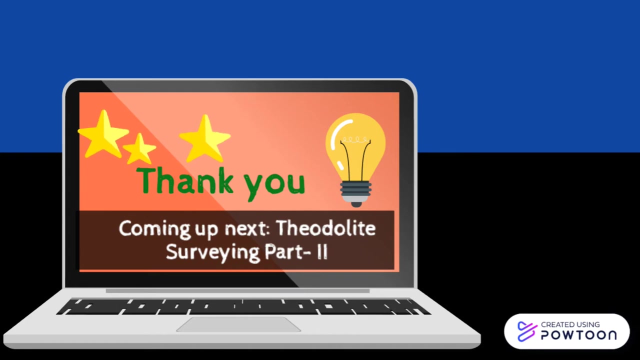 today we discuss the two basic functions of the theodolite. right in the next lesson I will explain to you the part of the theodolite and how to focus it to a target correctly. okay, have a good day. thank you very much for watching this video. coming up next is theodolite serving, part two. 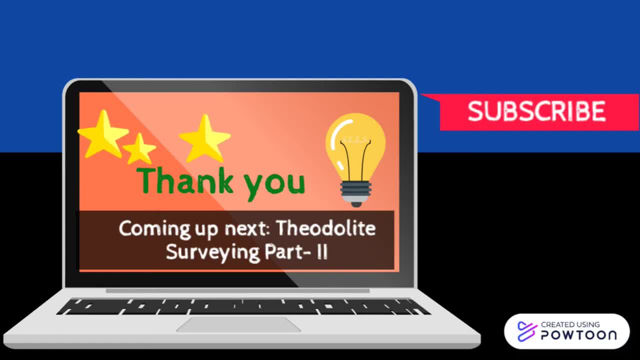 don't forget to subscribe this channel for more of the very latest videos.